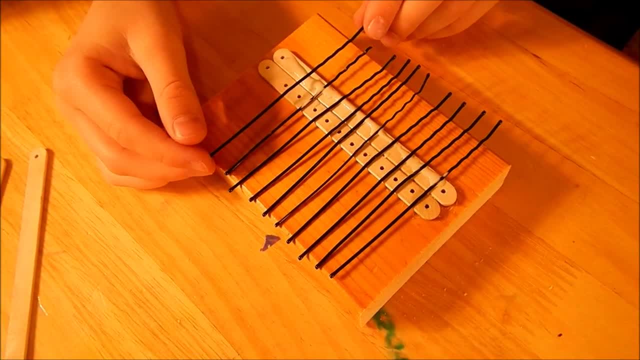 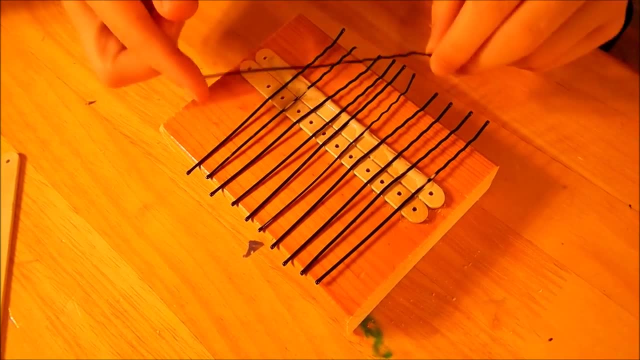 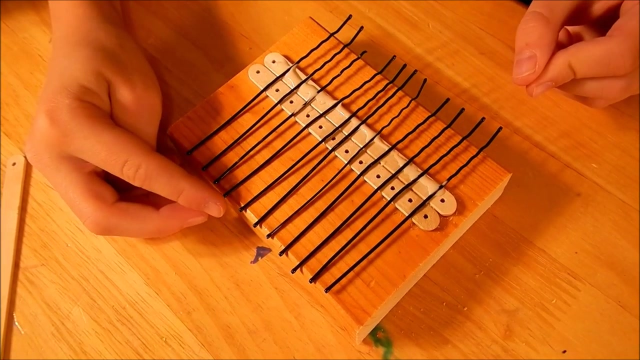 you want to take your time because the glue would put them down, but it will be really easy to hit the next one and it will like and they will all be like in one. that would be very, it would be like all crowded and I'll be bad and the way we're gonna have them be right on the edge. grab the. 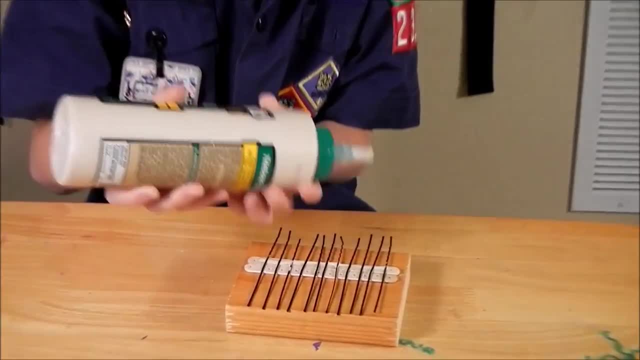 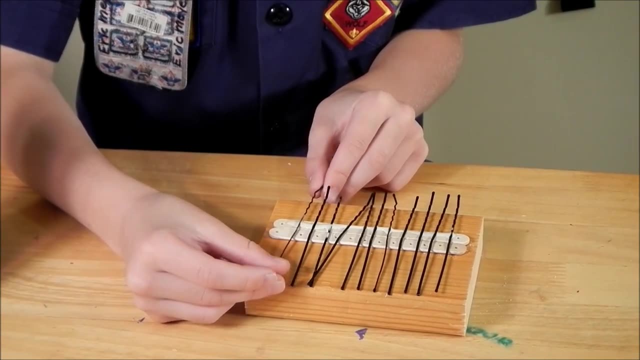 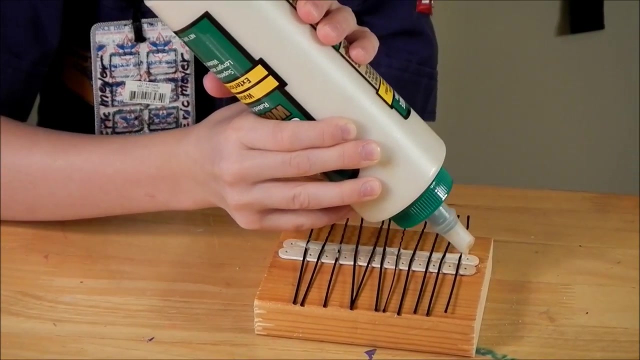 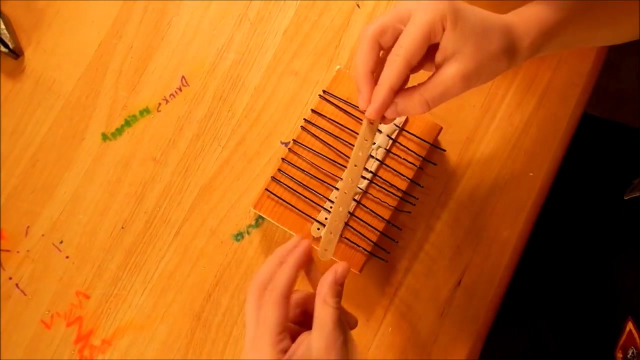 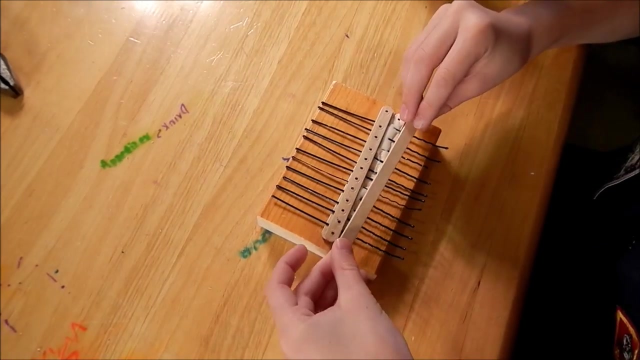 glue and we're just gonna go across. see what I was talking about. so, guys, now we're just gonna grab these two popsicle sticks and we're just going to line them up and set them on. we're gonna grab the nails and we're just going to set them in between. 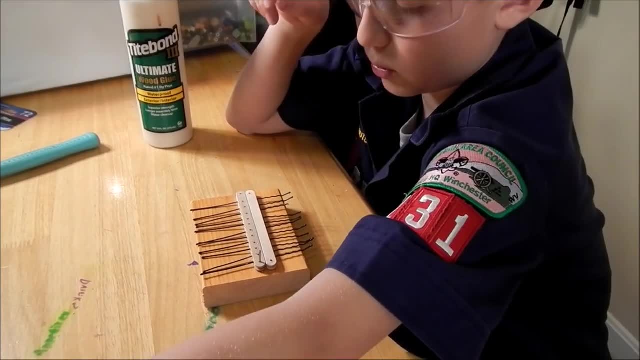 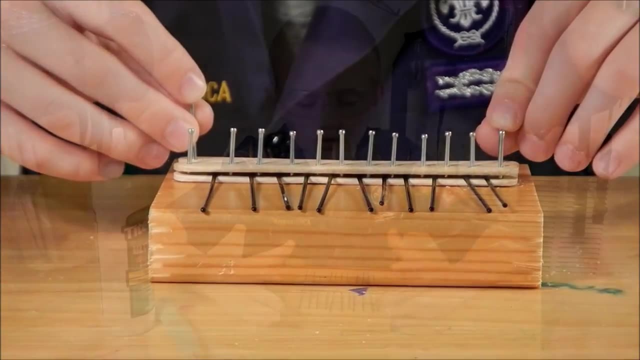 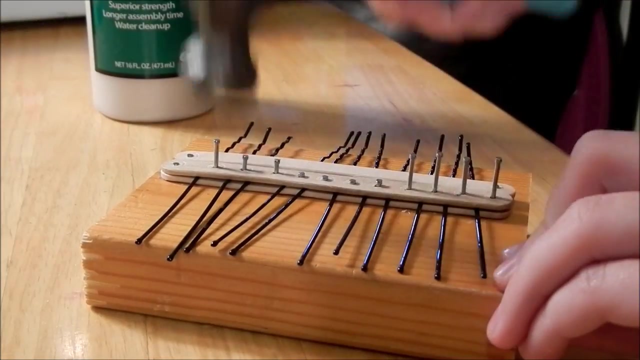 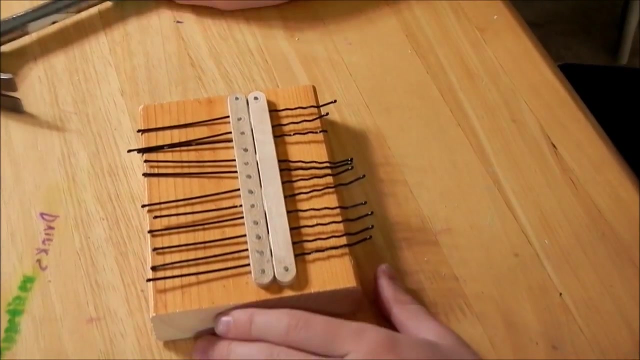 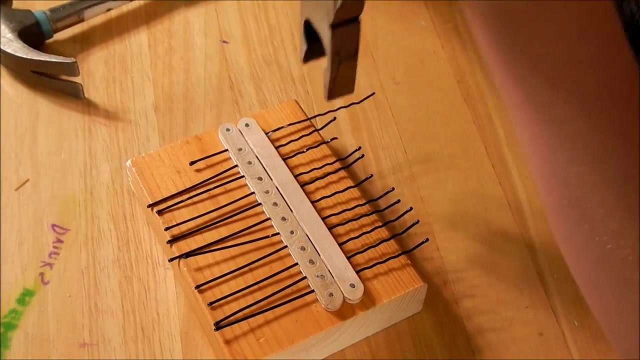 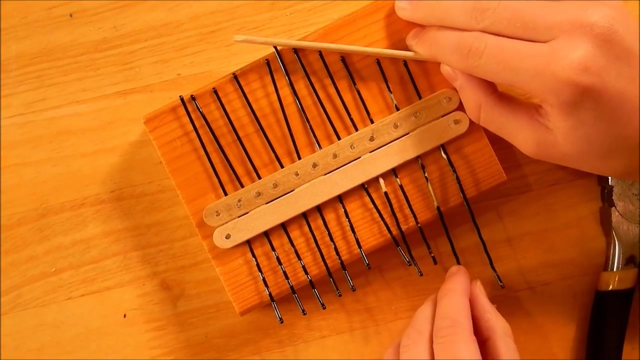 these. now you have to make sure the key in between each homes. you can't, we're just gonna pull them back. and if you can't pull them back And you're going to use the wires, We're going to grab our popsicle stick and we're just going to line it up so that they can touch the line. 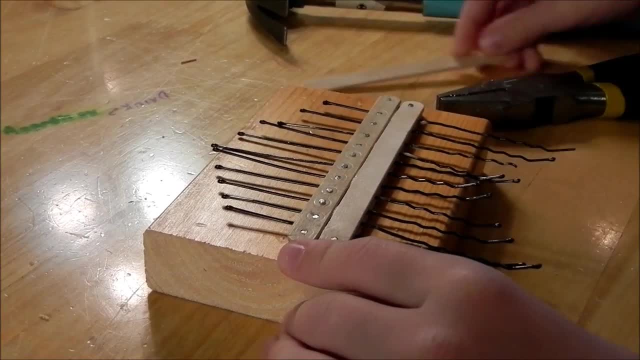 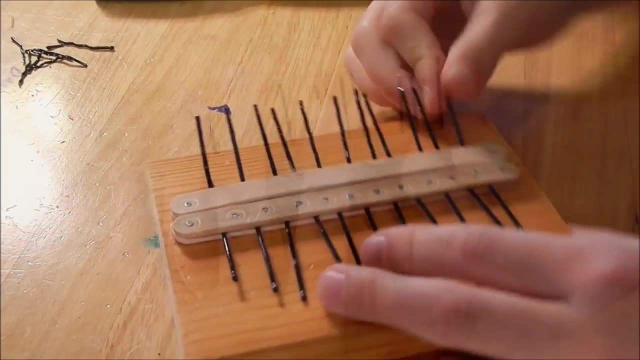 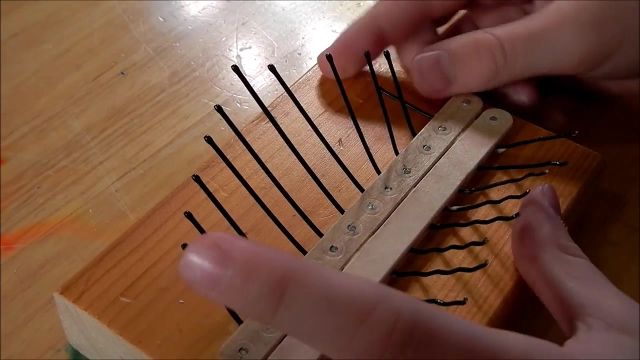 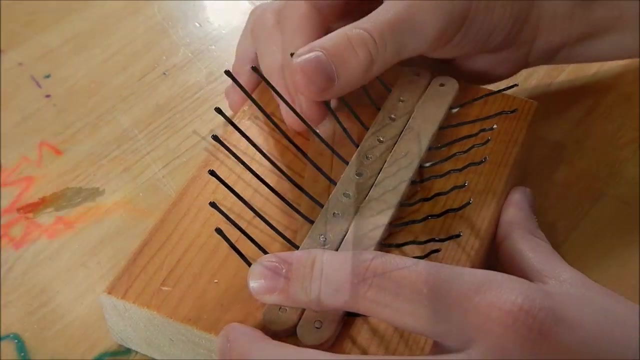 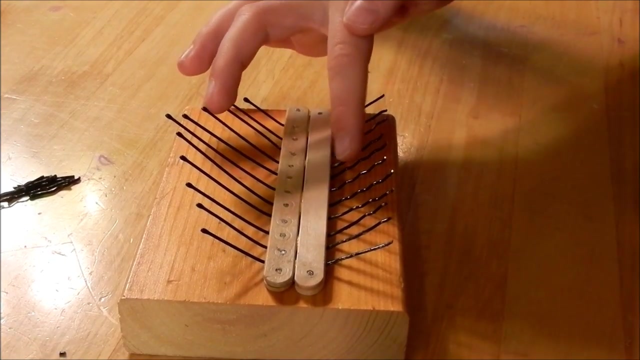 So, guys, now we just finished lining the bobby pins up. Now next step is we need to cut the bobby pins. So, guys, we'll bend them back to a 45 degree angle, And there we go. So, guys, once you finish straightening them up, you're going to grab your glue and you're just going to spray it all through on the tinier side, where you don't play on. 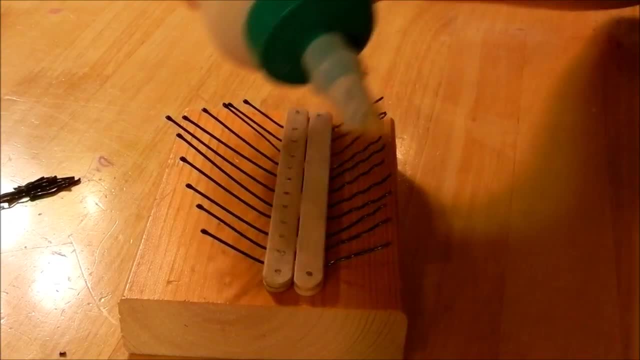 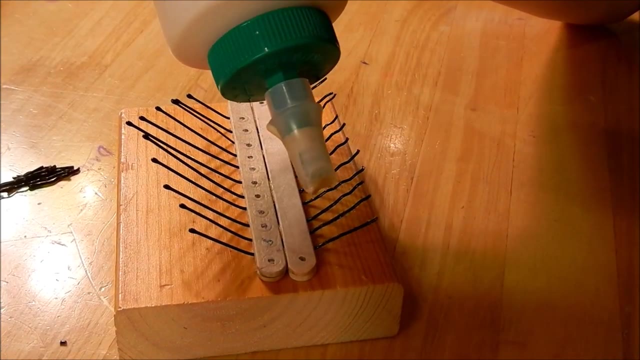 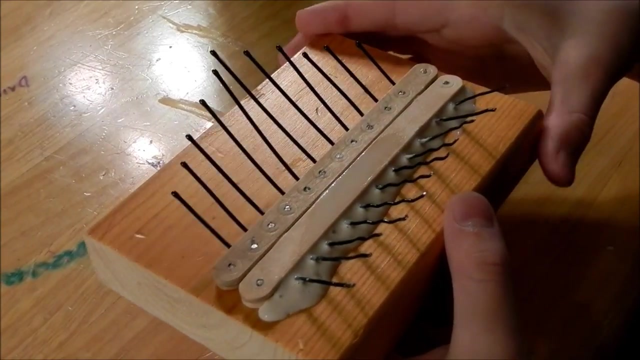 And if you use a glue gun It'll go way faster. But we're just going to do the normal glue gun. So, guys, you see why I put a lot of glue, Because it's going to help the keys stand, And now we're going to set this aside and let it dry for about one hour.